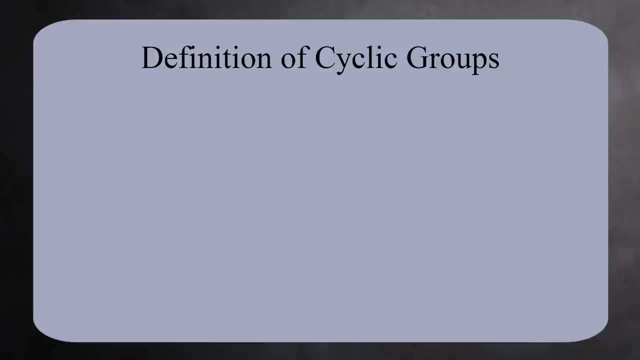 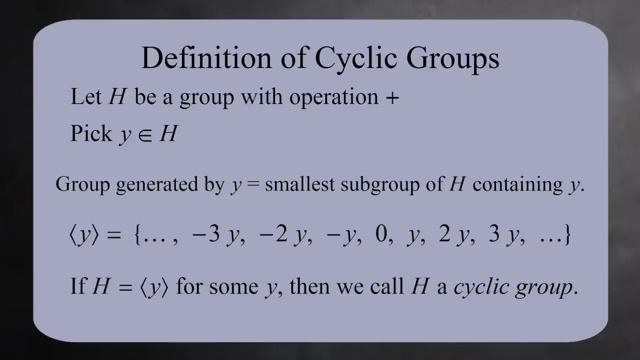 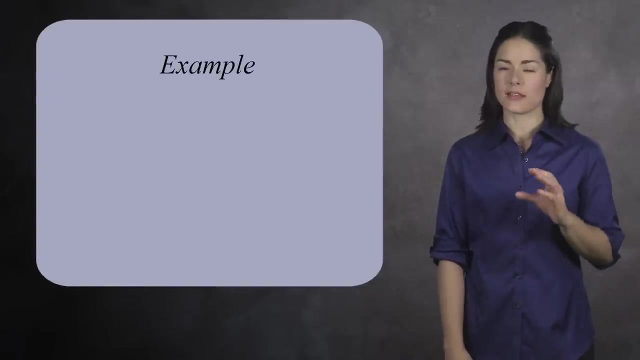 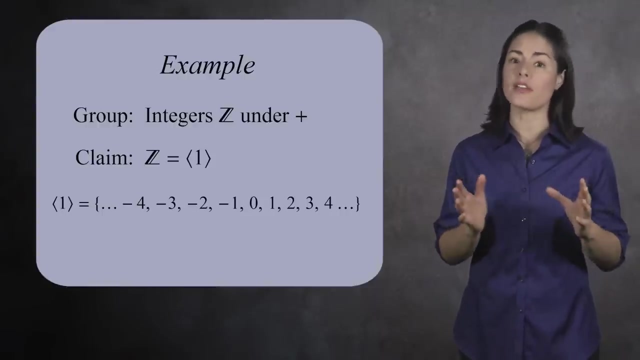 It's worth taking a moment to repeat this definition using additive notation. Let h be a group, and pick an element y in h. The group generated by y is the smallest subgroup of h containing y. It must contain y, its inverse, negative y, and the identity element 0. And to be a group, it must contain all positive and negative multiples of y. If h can be generated by an element y, then we say h is a cyclic group. Let's look at a few examples of cyclic groups. A classic example is a group of integers of x under addition. The integers are generated by the number 1. To see this, remember the group generated by 1 must contain 1, the identity element 0, the additive inverse of 1, which is negative 1, and it must also contain all multiples of 1 and negative 1. This covers all the integers. The integers are a cyclic group. 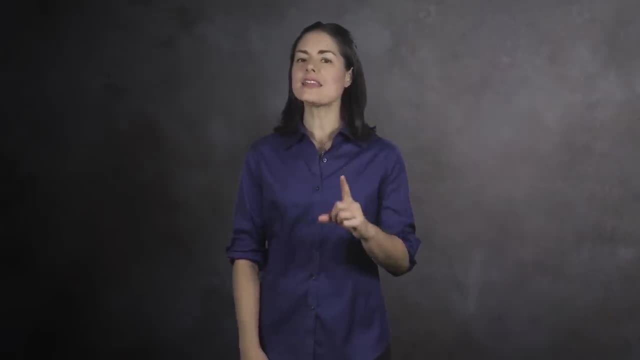 The integers are an example of an infinite cyclic group. Let's now look at a finite cyclic group. 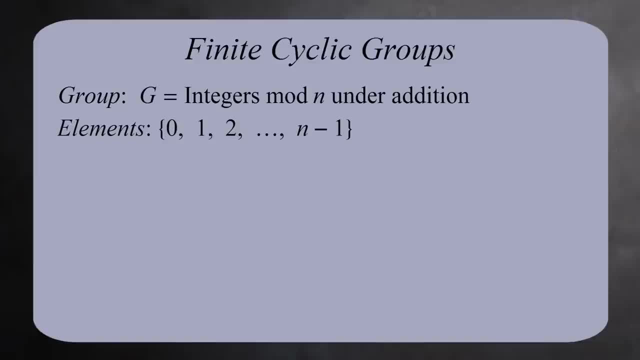 This is a finite group with n elements. It is also generated by the number 1. But something different happens here. Look at all the positive and negative multiples of 1. Recall that n is congruent to 0 mod n. n plus 1 is congruent to 1 mod n, and so on. Negative 1 is congruent to n minus 1. Negative 2 is congruent to n minus 2, and so on. So the group generated by 1 repeats itself. 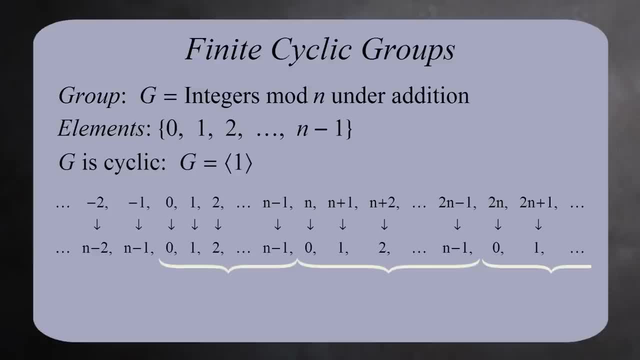 This is why it's called a cyclic group. 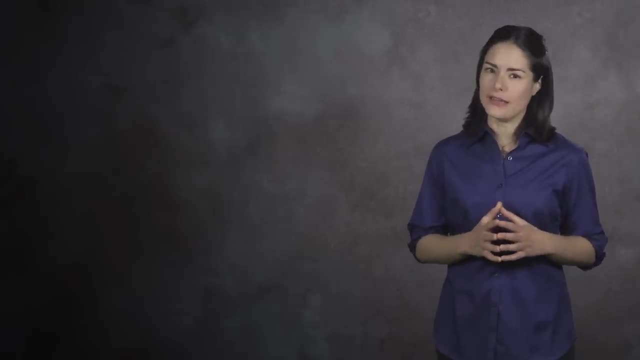 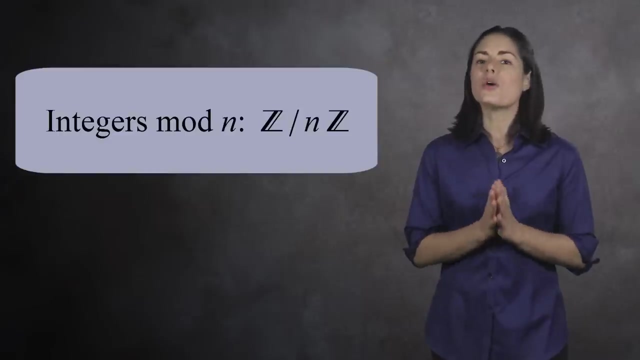 The integers mod n are a finite cyclic group under addition. In abstract algebra, the integers mod n are written like this. This will make sense once you've studied quotient groups, so don't panic if you're not familiar with this notation. 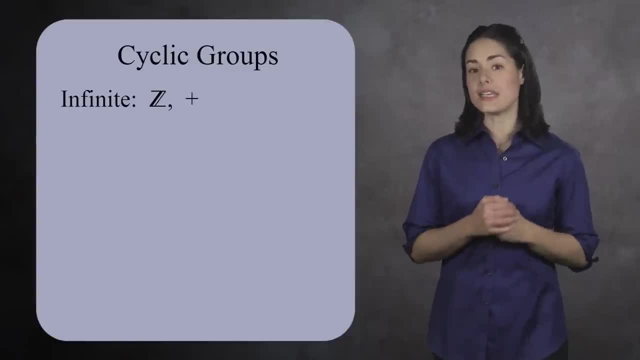 We've now seen two types of cyclic groups. The integer z under addition, which is infinite, and the integer mod n under addition, which is finite. 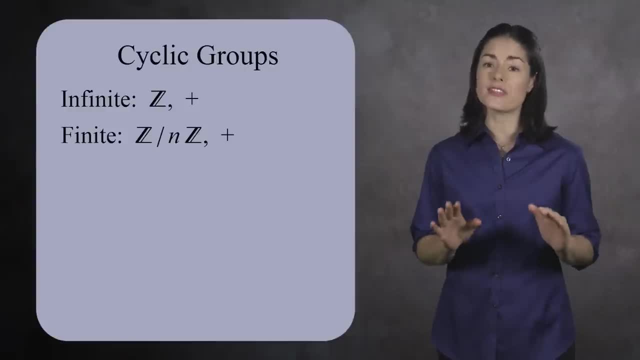 Are there other cyclic groups? No. This is it. The complete collection of cyclic groups. 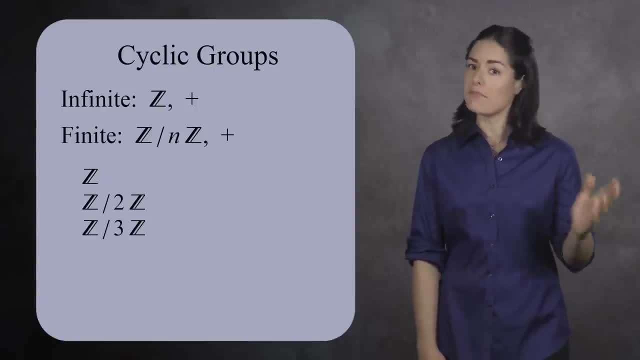 The integers, the integers mod 2, the integers mod 3, the integers mod 4, and so forth. Oh,